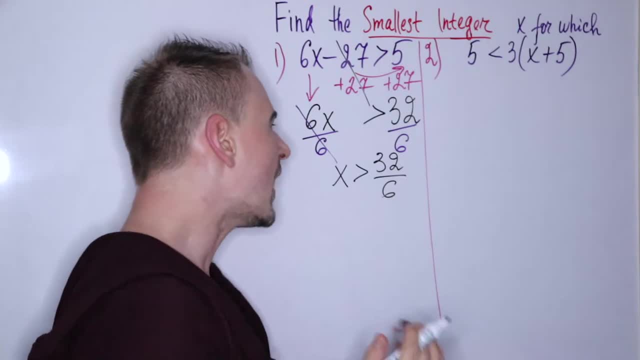 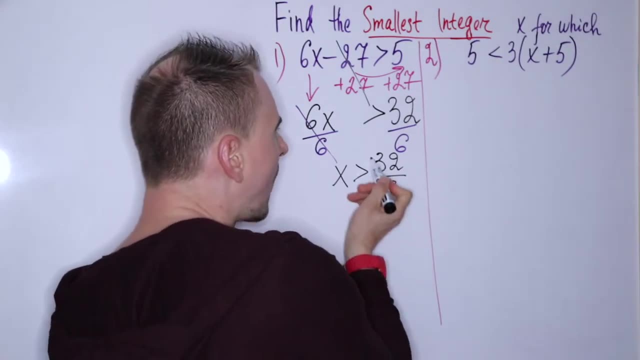 so try to reduce it as much as you can. So at least they both, both of them divisible by 2.. So try first of all reduce it by 2.. So 2 goes into 32.. 2 goes into 32, 16 times. 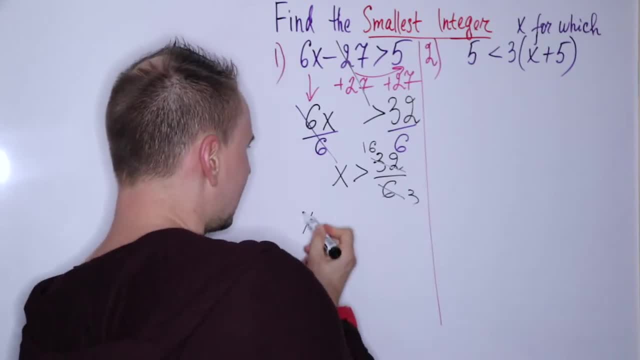 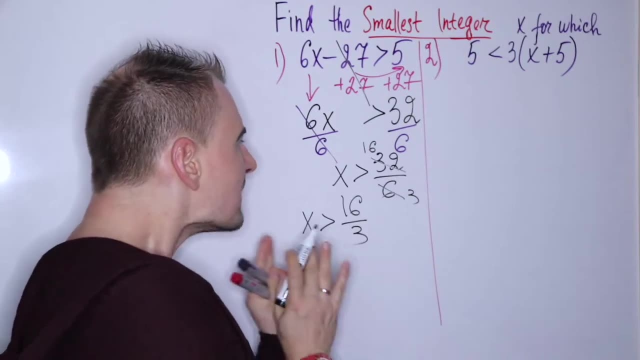 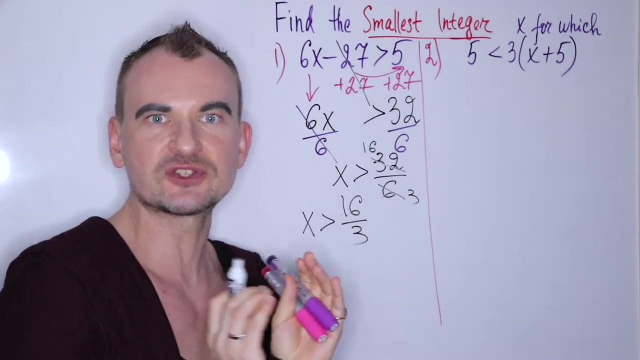 And 2 fits into 6, 3 times, So you would be left with x greater than 16 over 3.. Now, basically, this is a solution set for this inequality, And always keep in mind so when you solve an inequality. 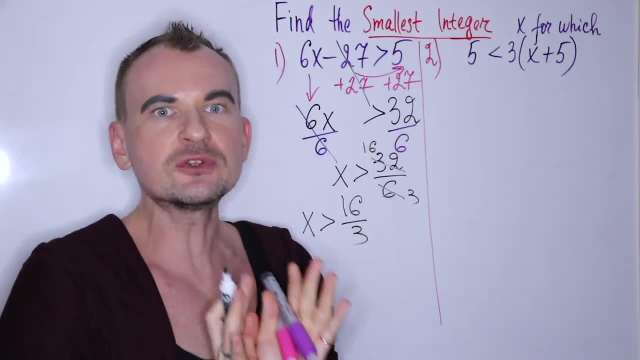 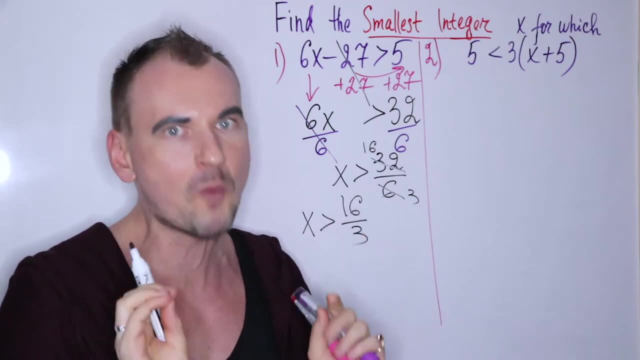 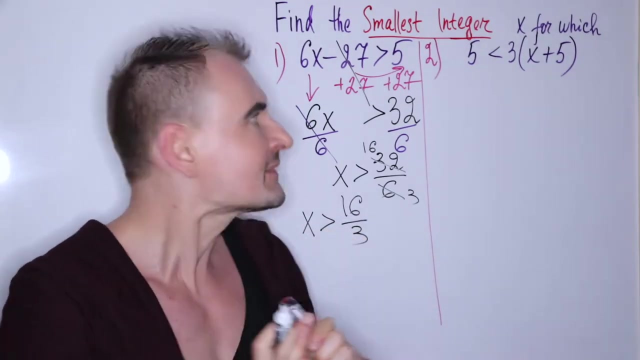 your answer, your solution set. if it comes to solving your solution set, your solution is always a solution set. So basically, it's an infinite set of x that work for your inequality and satisfy your inequality. in other words, Now, since we are not kind of interested in finding a solution set, 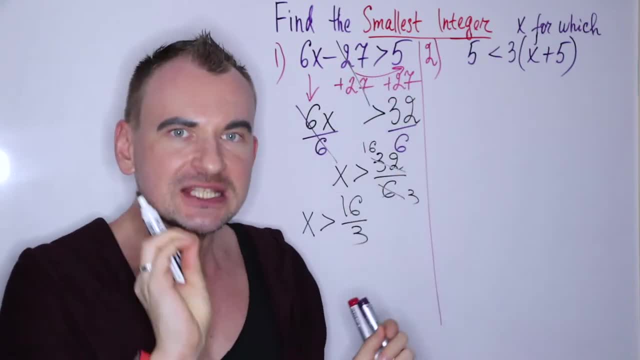 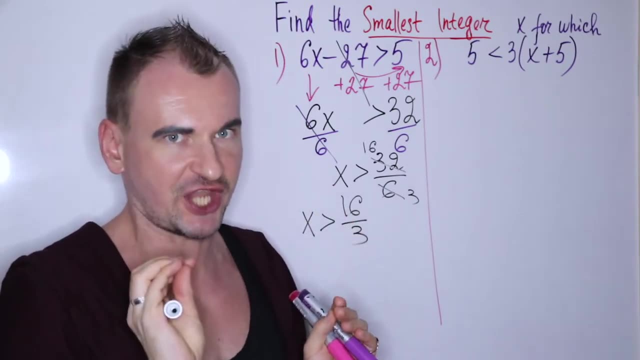 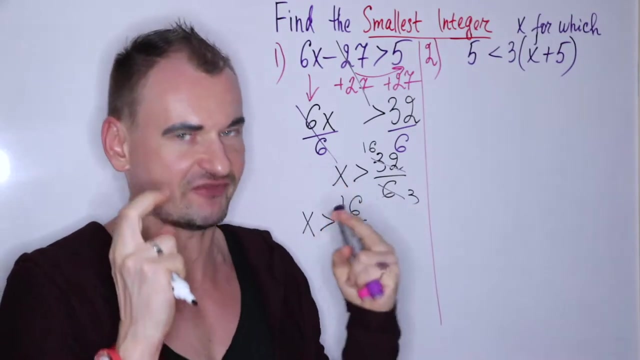 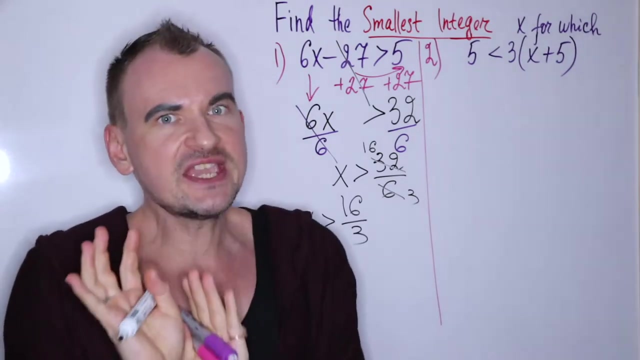 but we have to find the smallest integer that basically, in other words, belongs to your solution set. So satisfying your inequality means your smallest value of x, smallest integer value of x, belongs to your solution set. Now, what are the integers? So keep in mind that integer numbers, they are basically all natural numbers. 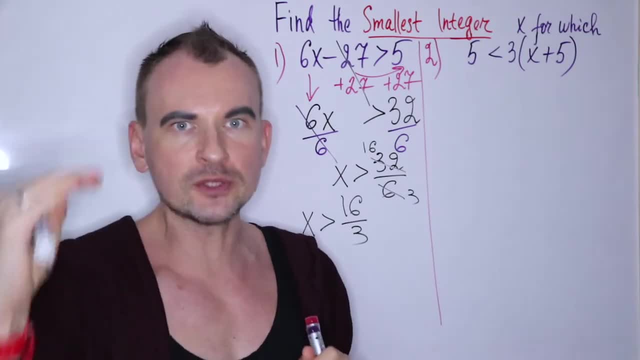 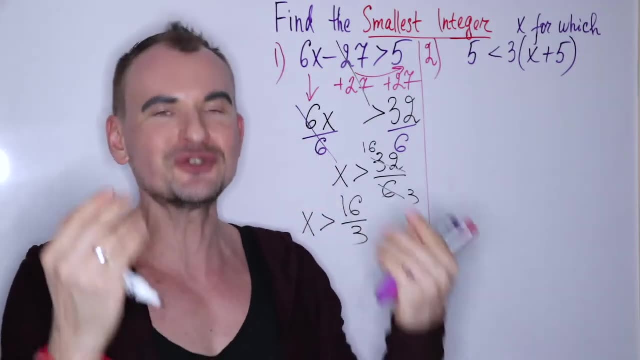 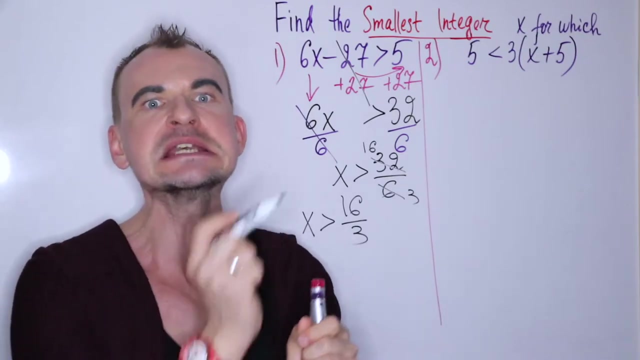 So 1, 2, 3 keeps going on on on including 0. So you throw in 0. And also you take the negatives, So you take the opposites to this natural number. So basically it's negative 1, negative 2, negative 3.. 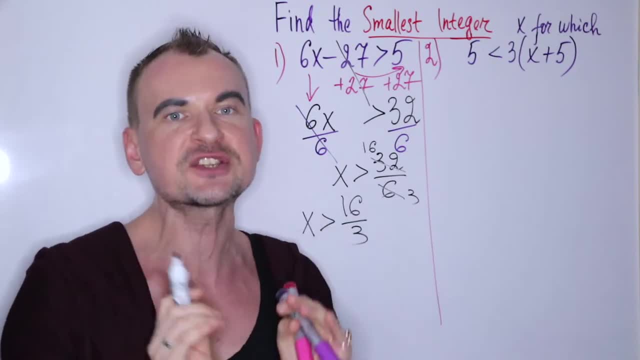 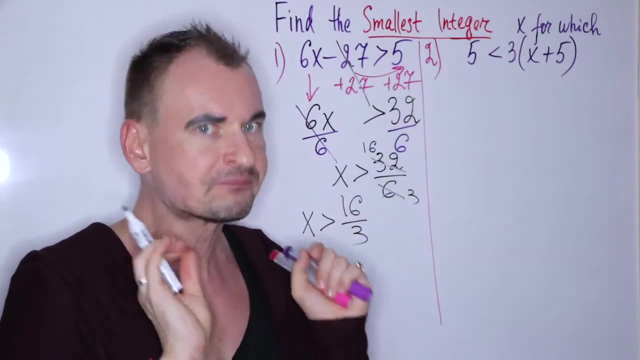 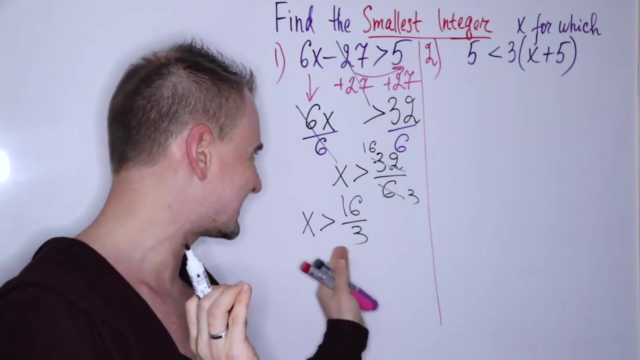 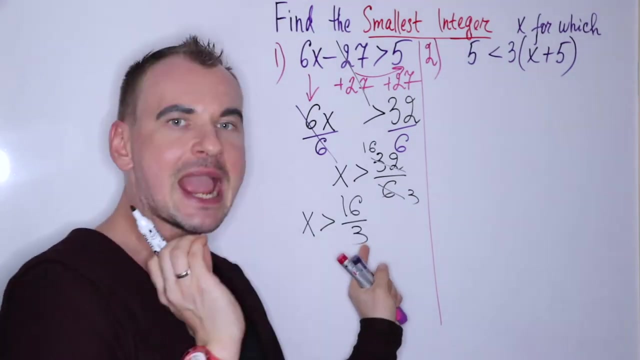 So, all of these numbers, all of this set of these numbers, they form, they give you the set of integer numbers. So, basically, what we are looking for, We are looking for the smallest integer number that satisfy, that satisfies this inequality. So, since it happens to be in improper fraction, 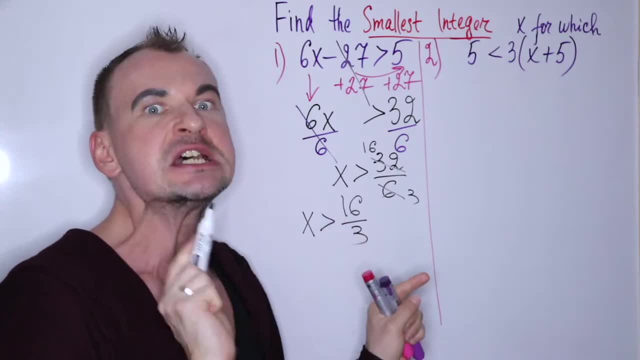 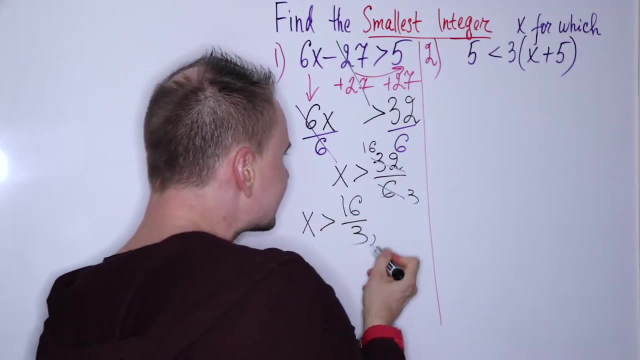 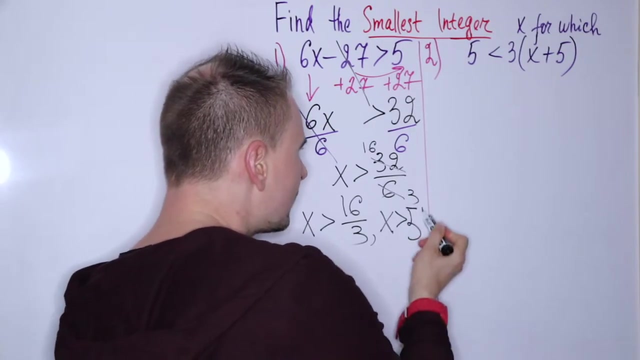 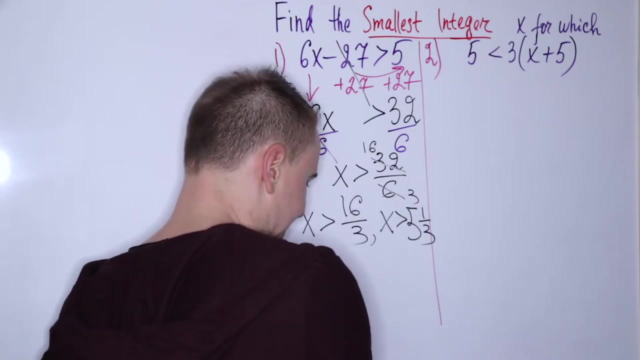 so your top number, your numerator, is greater than denominator. First of all, let's convert it, Let's turn it into a mixed number, So, since 3 goes into 16, five times, leaving you with 1 over 3.. So this one is going to be the solution set, basically. 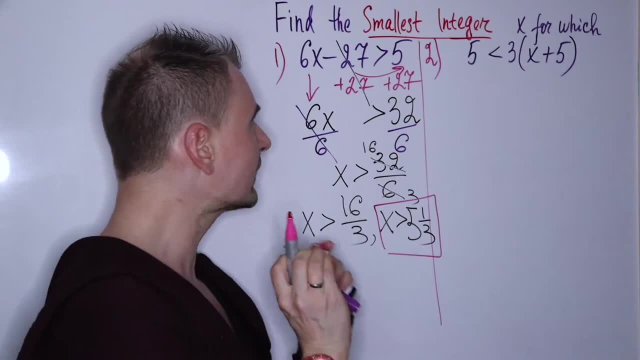 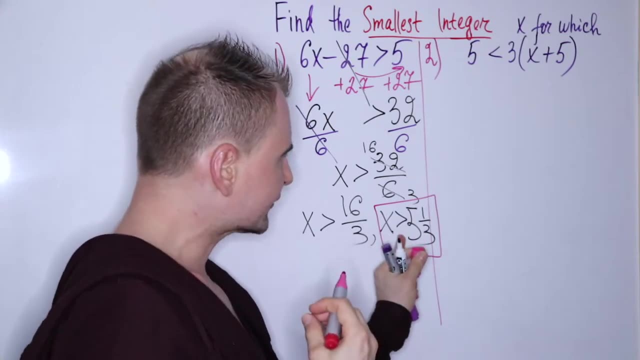 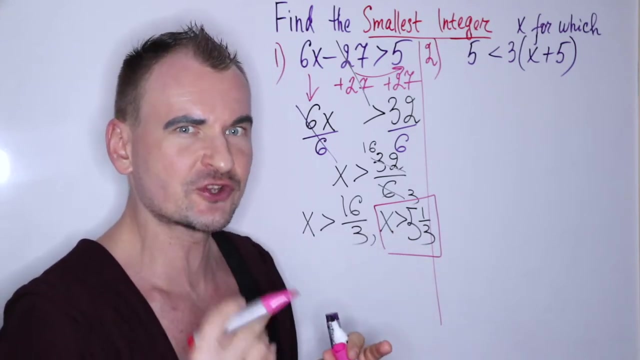 for this inequality. So we are looking for the smallest integer that satisfies this solution set And, if you look at this, so your x, your x, is basically have to be greater than 5 and a third. So the smallest value, the smallest integer value. 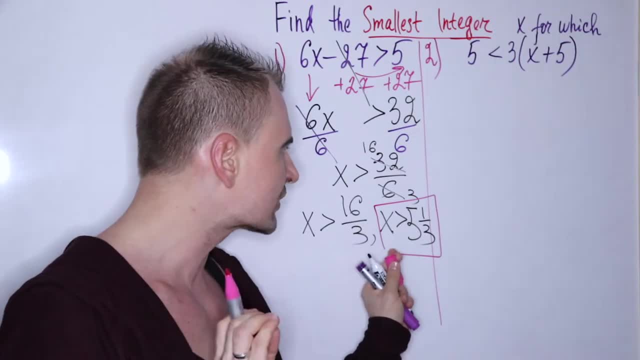 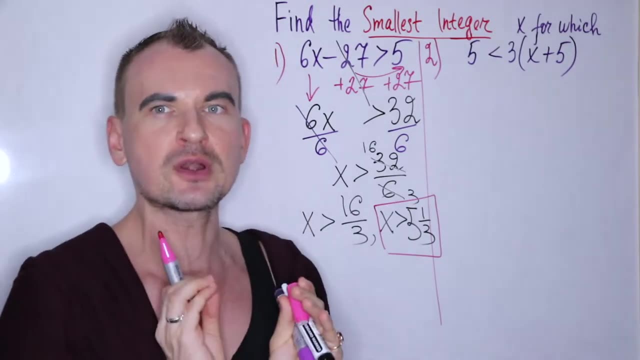 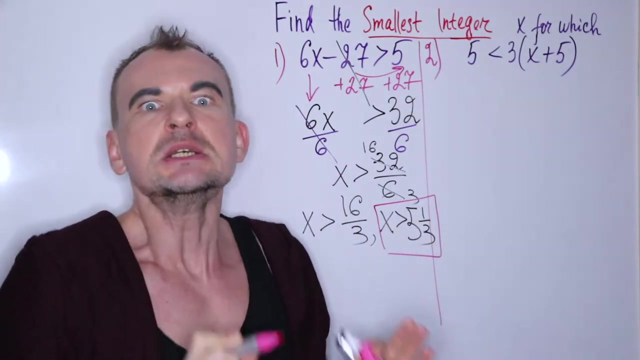 of x, for which this works, is going to be 6.. Well, if it's still difficult for you to figure out in your head for all of these problems, you could always draw a number line and you could represent your solution, set on this number line and take this figure out. 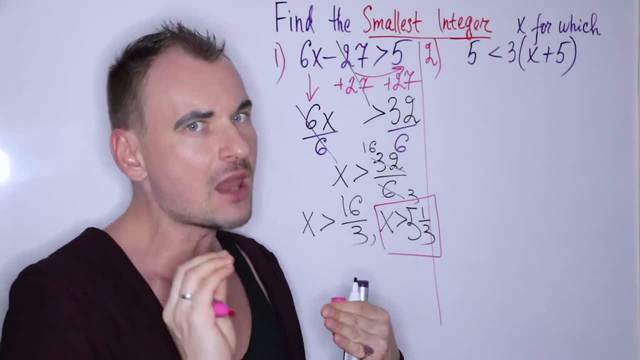 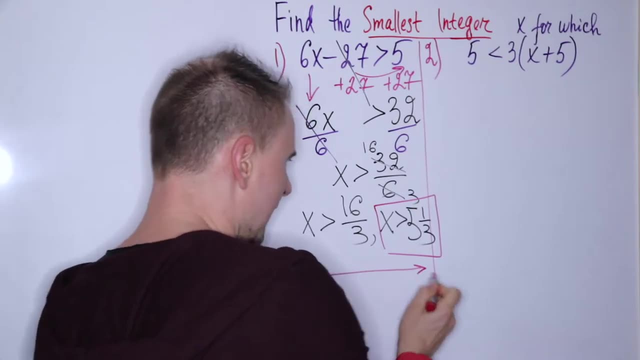 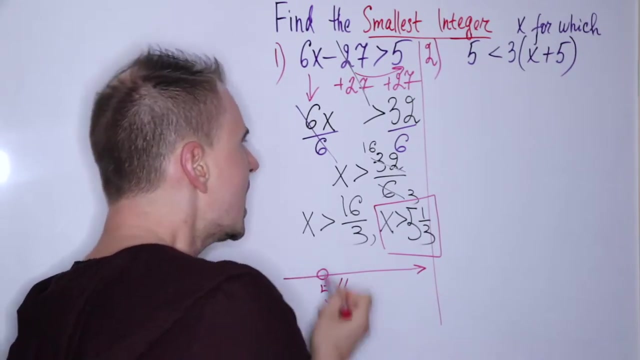 work out the smallest integer from a number line, if it helps. So let me do it quickly. So you draw just a number line. You are going to place this value, 5 and a third, on your number line And your solution set, or your axis. 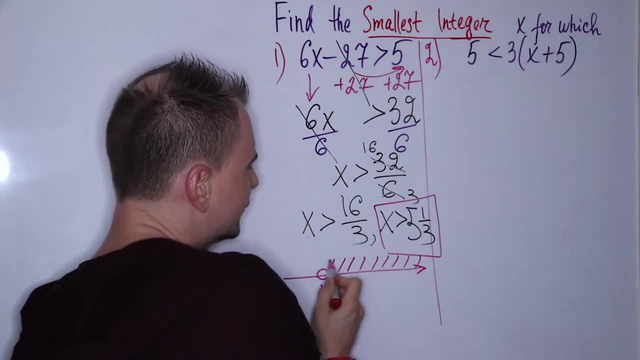 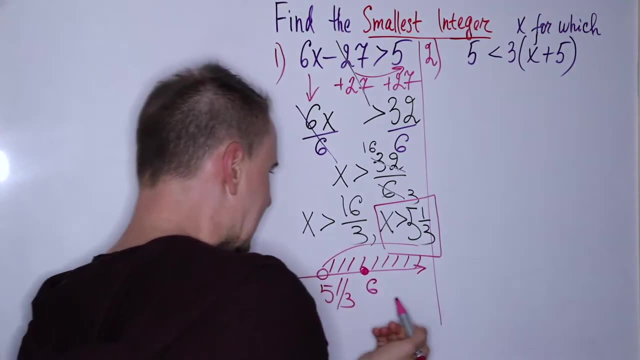 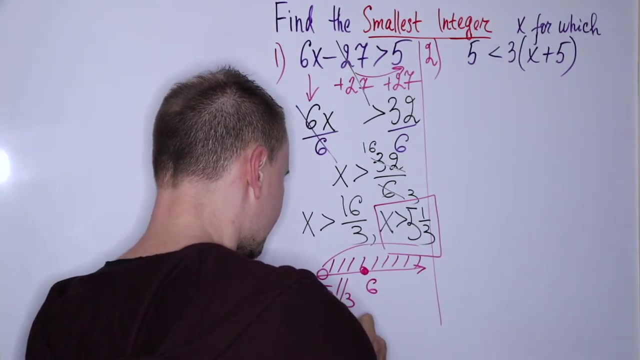 is going to be greater than this value. So we are going to this right direction. The smallest integer is going to be 6, since basically your 5 is on the left. So the smallest- and we could write it down- the smallest value of x is going to be 6.. 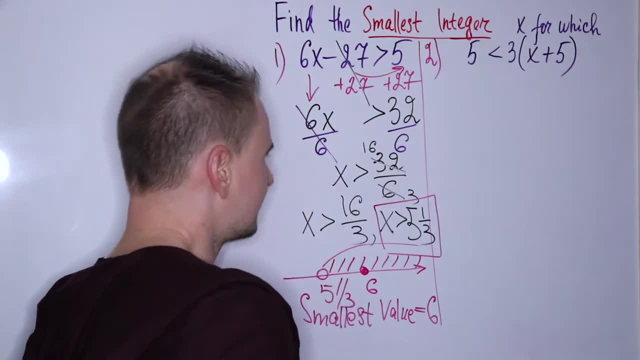 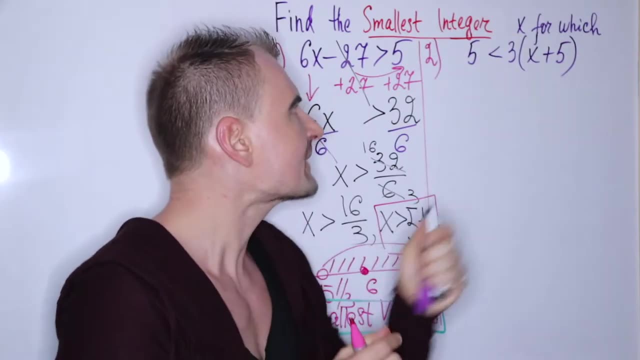 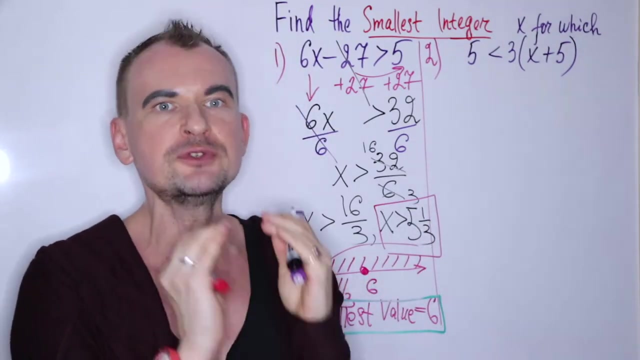 So that's basically answer. So that's basically what you asked for. Now say, you have been given something like this: Well, it's similar, likewise, but you have the parentheses. So first of all, you need to get rid of the parentheses. 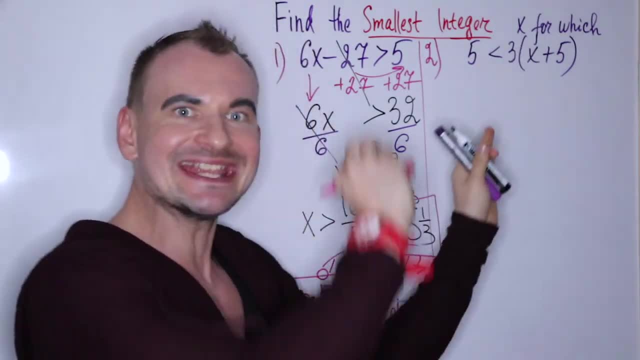 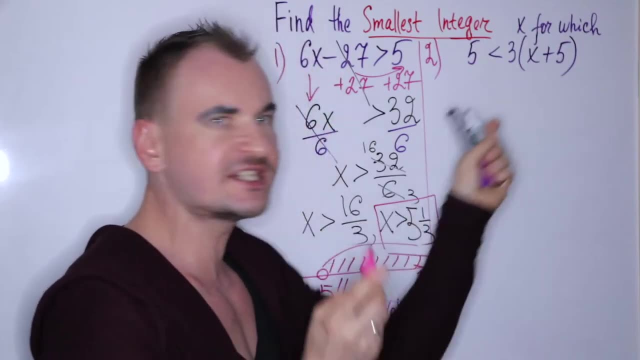 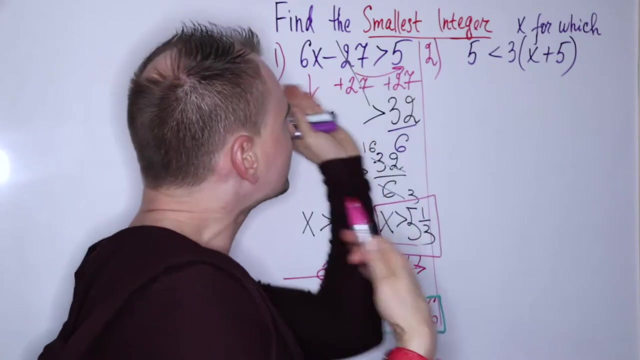 So remove them. So by taking these three and distributing over whatever you have inside, And basically you are given this inequality in a kind of reverse order. So for me it's not that natural. I'm used to this way of solving. 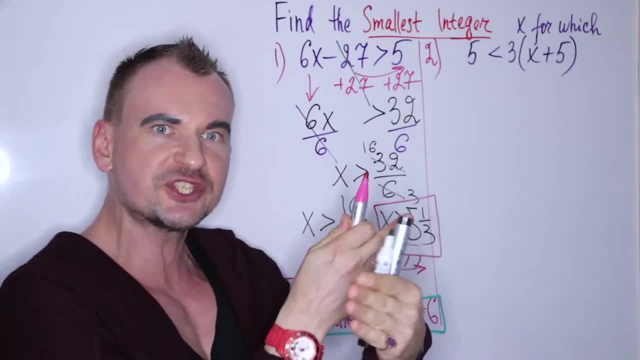 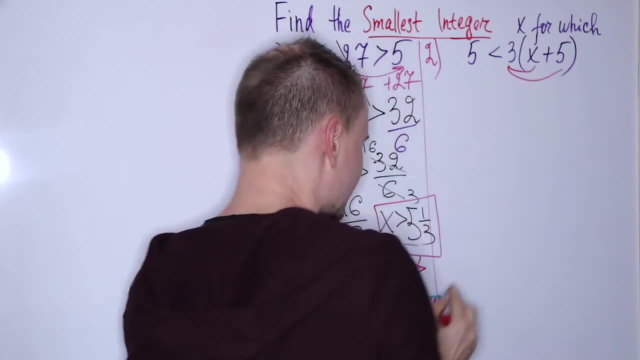 of writing inequality. So also I'm going to switch, I'm going to swap the order. So again at this point I'm going to distribute these three and apply to both terms Inside the parentheses. So in the next line on my work. 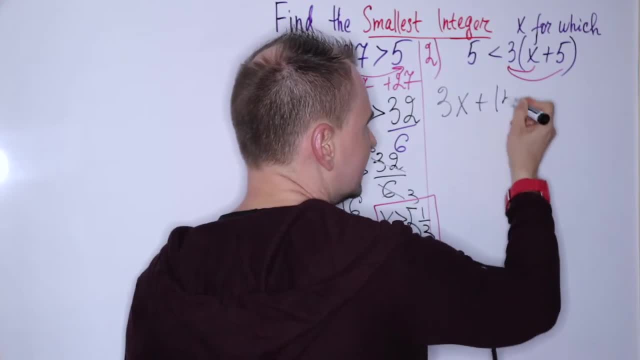 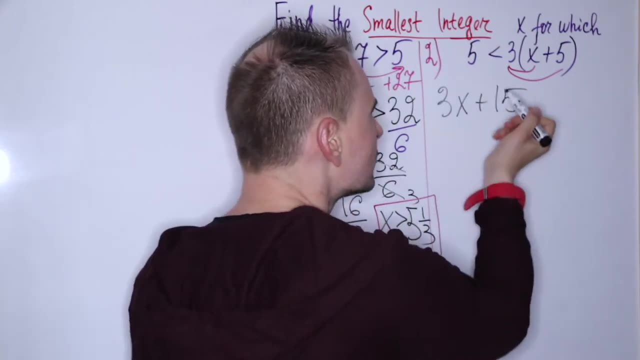 it becomes 3x plus 15.. So we opened up, we remove, we distribute these three, we fold it out, we multiply it out, And I'm going to write it in the reverse order, as I said. So it's greater than 5.. 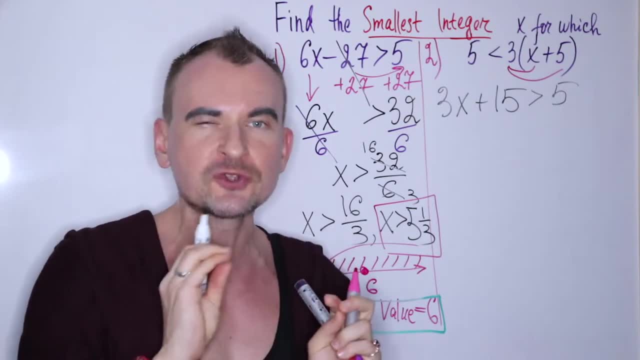 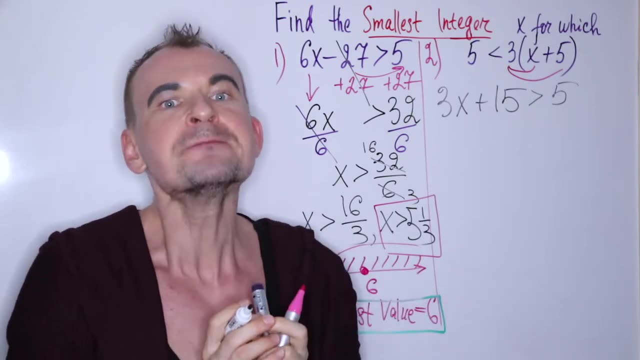 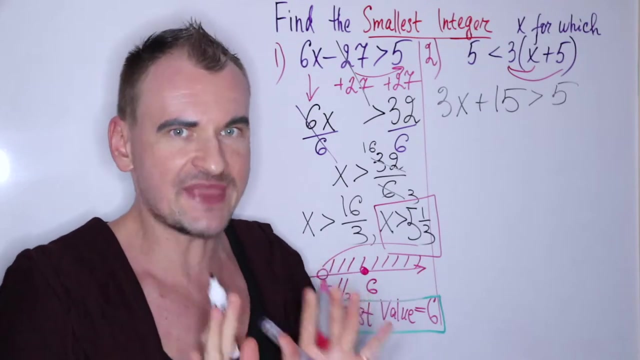 And, by the way, I have a bunch of videos on solving linear inequalities And if you need a help with solving linear inequalities, you could use the link down below in the description box and check it out for that explanation. Now, in the same way, similarly. 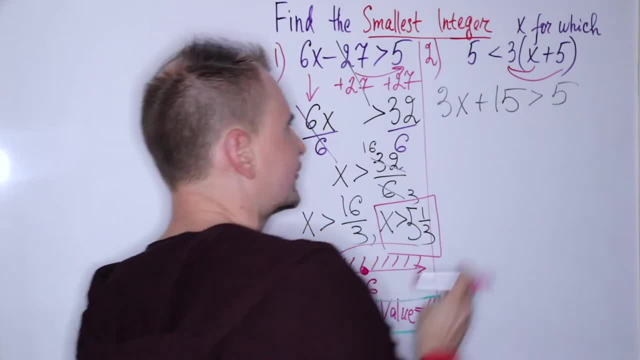 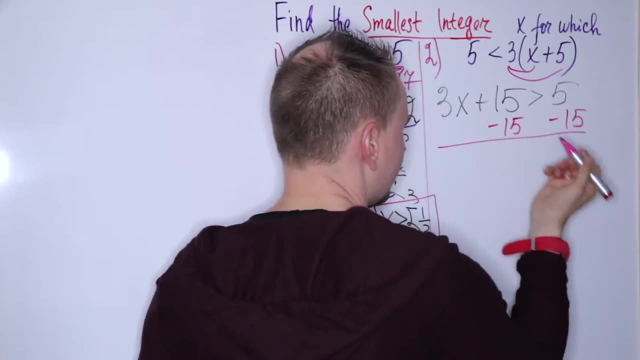 so I want to move this 15 to the right side by taking this 15 off, taking it away from both sides of your inequality. So 15 goes away, disappears, drops out. So bring down this 3x at this point. 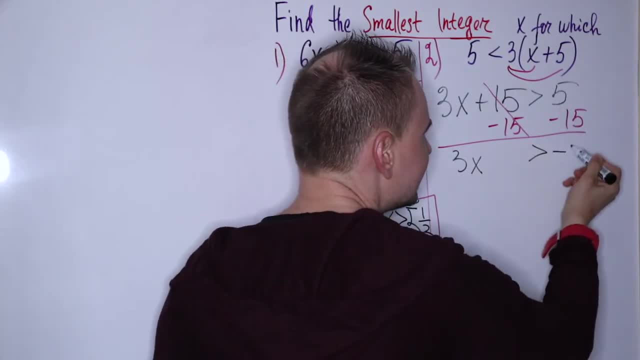 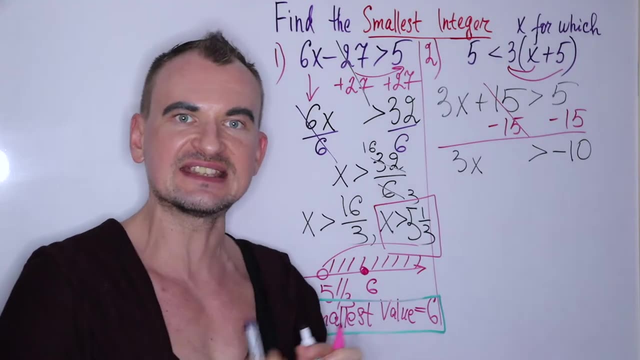 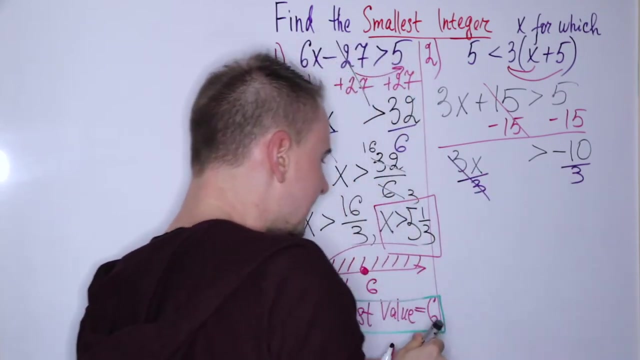 greater. 5 minus 15 gives you negative 10.. And again, at this point, whatever the issue is, in this case it's 3, divide through, Divide through both sides of your inequality, So you divide by 3.. So 3 goes away, disappears. 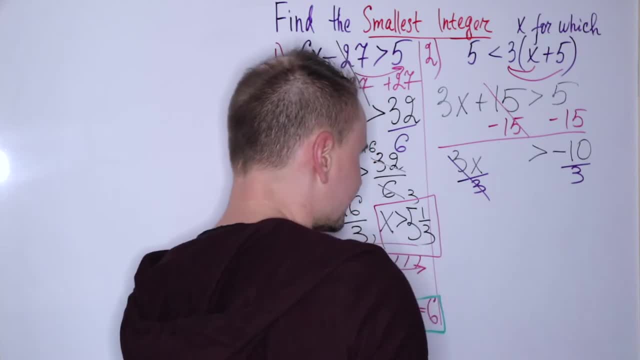 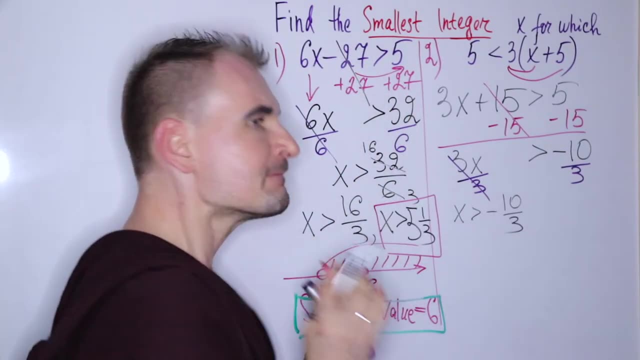 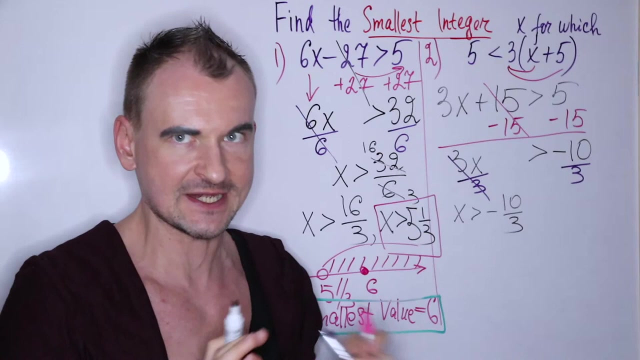 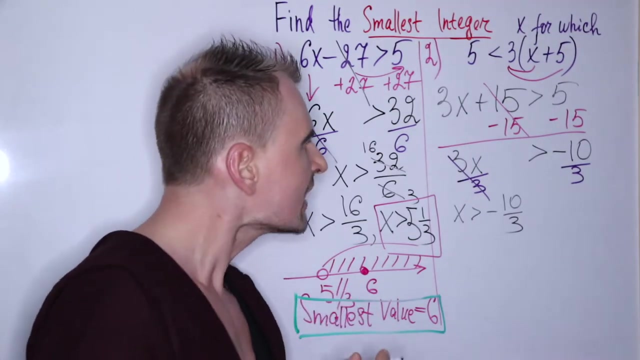 and you end up getting x greater than negative, 10 over 3.. Again, at this point, this is a solution. You can do that for this, for that given inequality, But since we are looking for the smallest integer that works for your inequality, 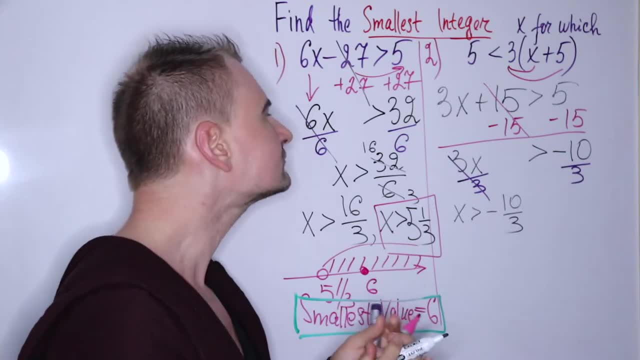 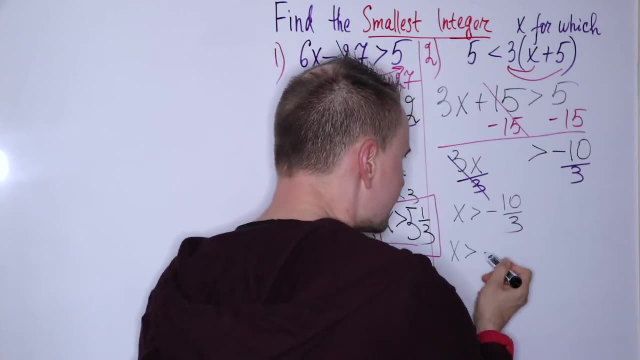 first of all, let's turn it, let's convert it into a mixed number, since it happens to be an improper fraction. So it becomes. so you keep this. negative 3 goes into 10,, 3 times, leaving you a field. 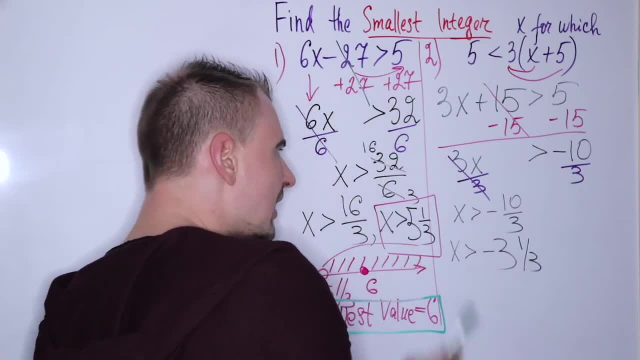 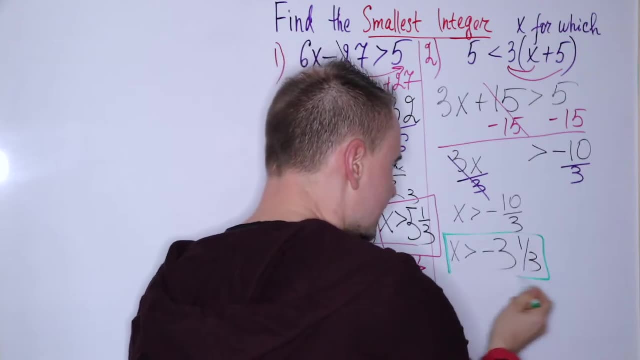 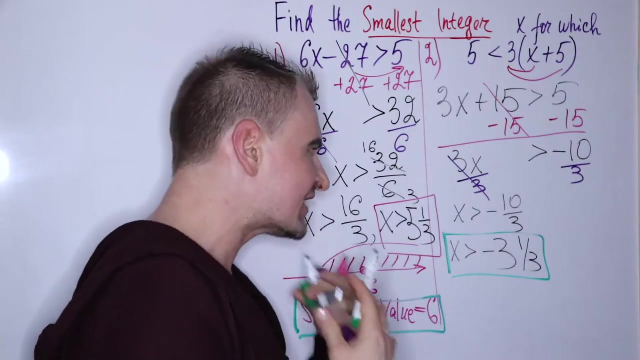 Now it's kind of similar what we had before, But the problem is we are dealing with negative numbers And you have to be careful with this, So it has to be taken with exceeding care. So and again, if it's still difficult for you, 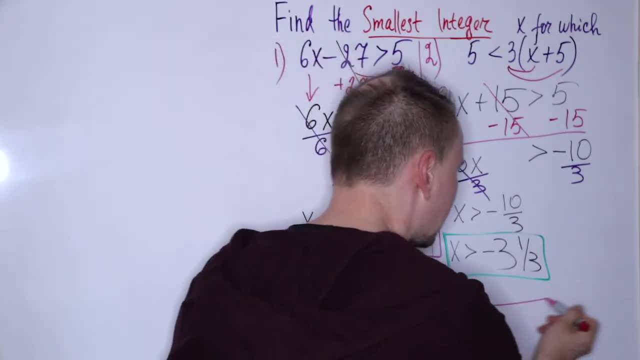 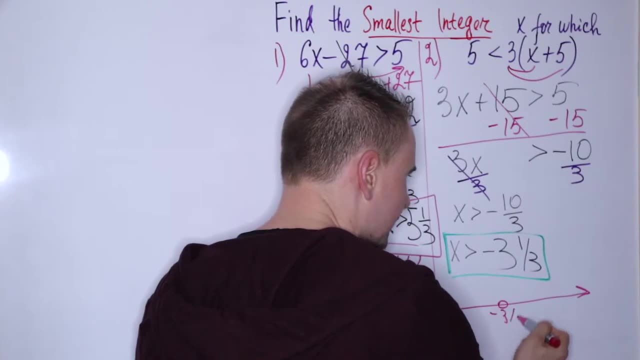 you could always draw a number line and place your solution set on a number line. So let's say you have this negative 3 and field somewhere And again x greater than so. we are going to this direction, But again, since we are dealing with the negative numbers, 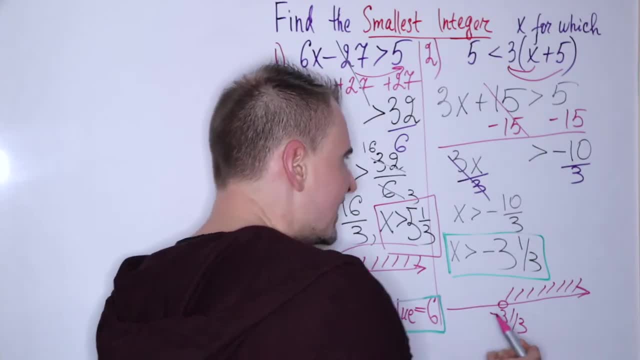 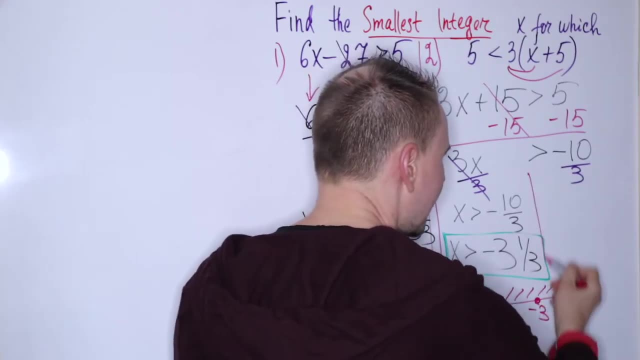 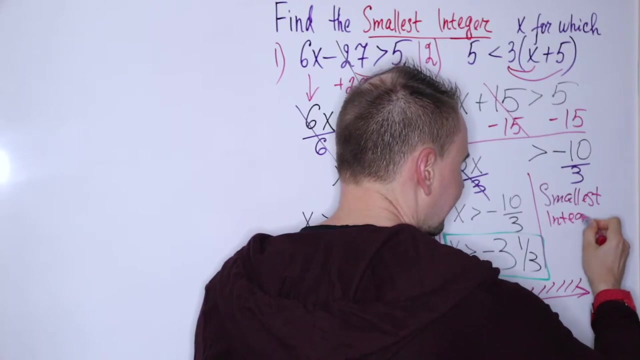 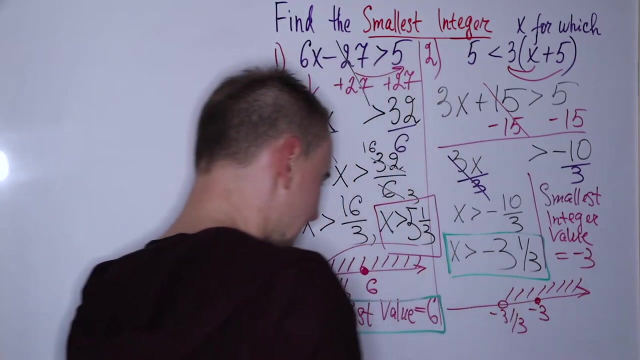 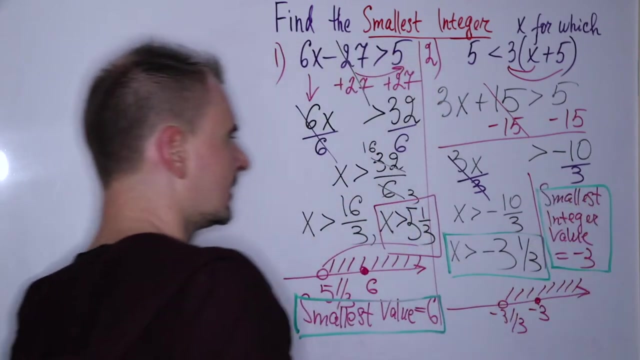 so your smallest value of x that satisfies your inequality is going to be negative 3.. So negative 3 is your smallest integer value, Smallest integer value. So it's going to be negative 3.. And that's your answer for that second inequality. 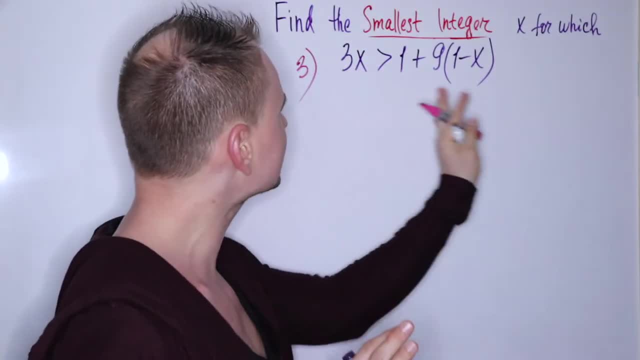 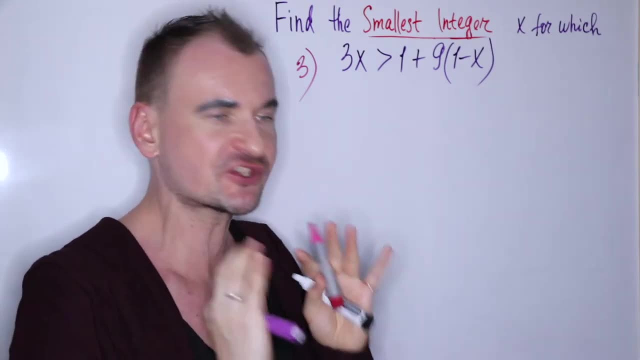 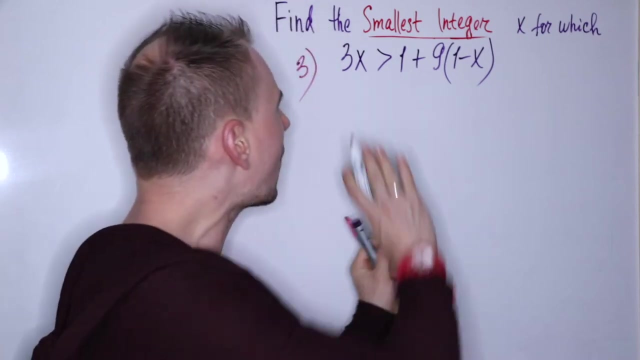 Alright, the last one. Suppose you have been given something like this, The same idea. So, first of all, the first thing to do is just normally solve your inequality. Alright, look at this. You have again parentheses on the right side. 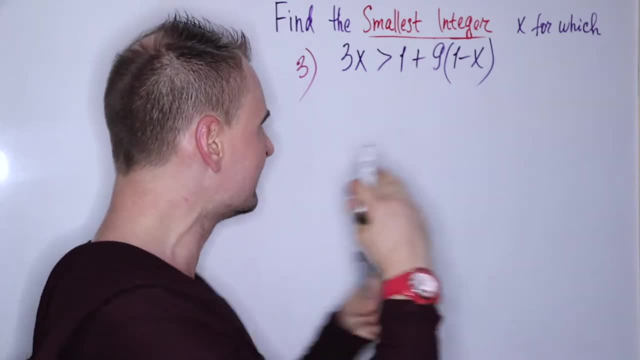 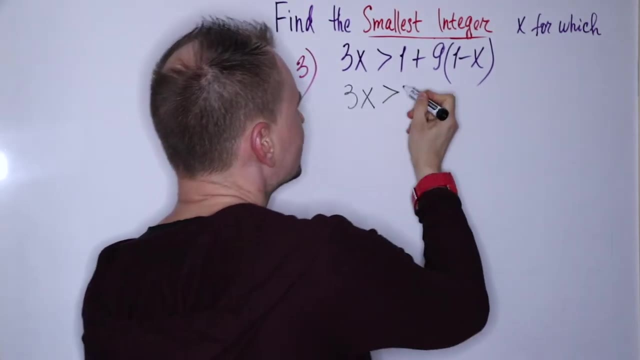 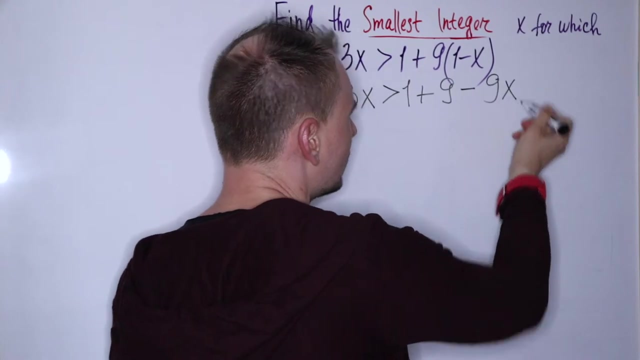 So, first of all, let's open up the parentheses, Let's remove it. We're going to rewrite left side as this: So 3x greater, So 1 plus. so 9 times 1 gives you 9,. minus 9 times x gives you negative 9x. 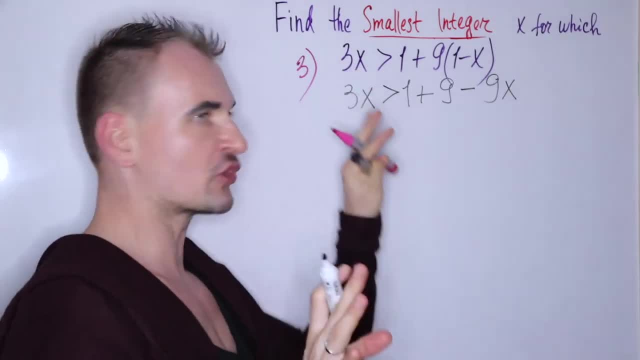 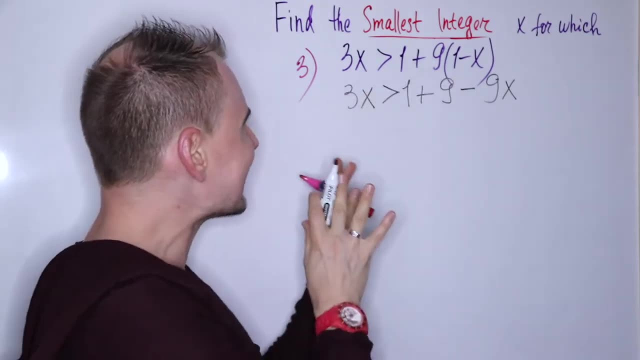 And again at this point you want to collect your x terms on one side of your inequality and your numbers, your constant, on other side, Since it's kind of little bit messy. so your terms and your numbers, they're like scattering around. 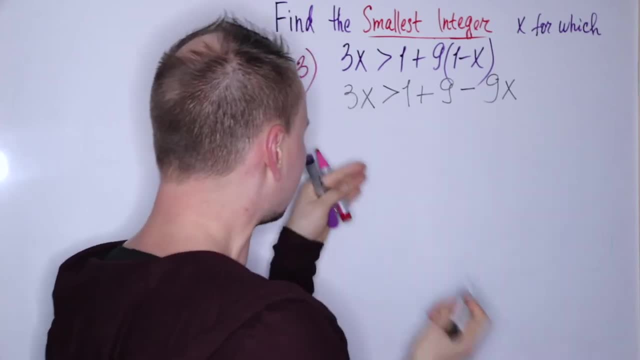 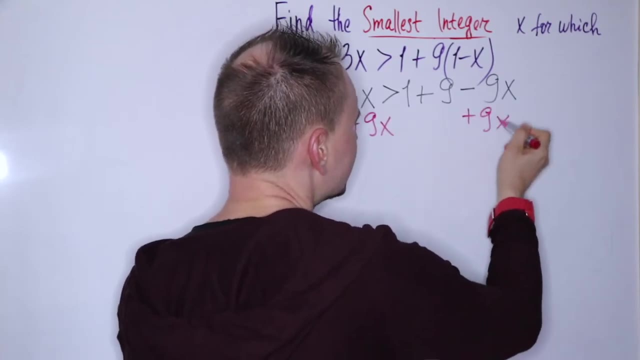 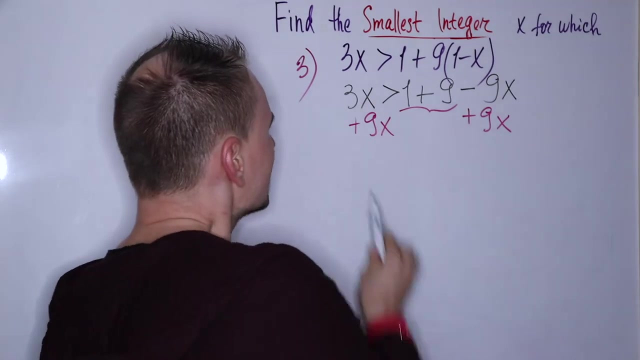 So bring this 9x first of all to the left side, by adding 9x to both sides of your inequality, And basically we can combine this one And 9, so that would give you just 10.. So 3x plus 9x. 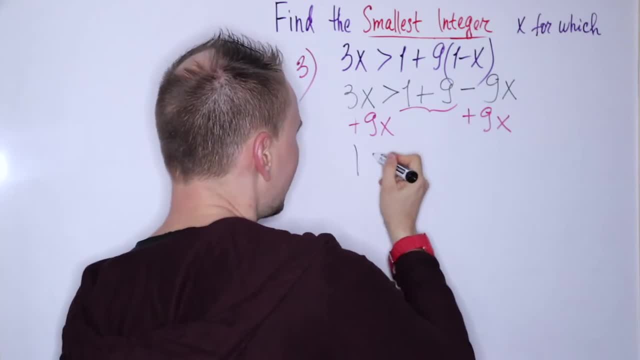 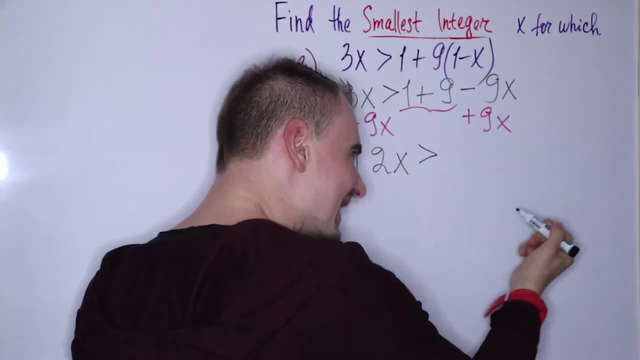 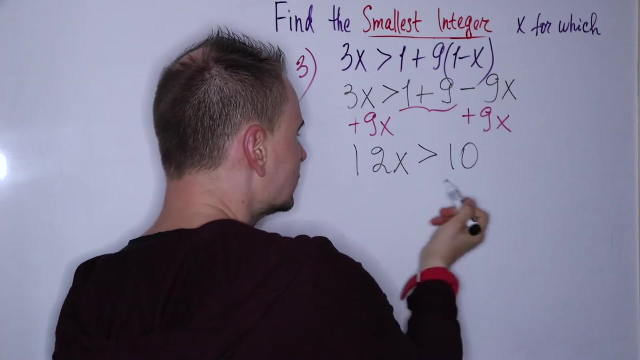 that gives you 12x. Bring down greater sign And on the left, on the right side, you end up getting just 10.. So now you want to isolate your x. Whatever takes, your x at this point is 12.. 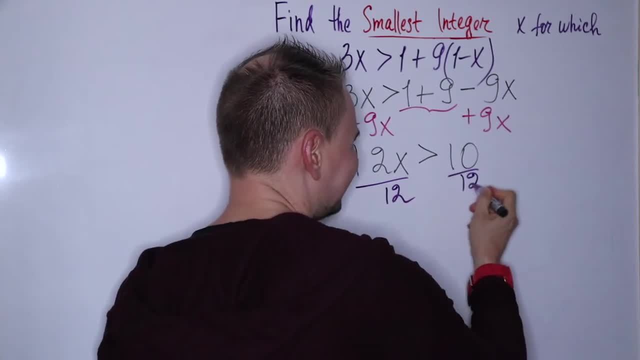 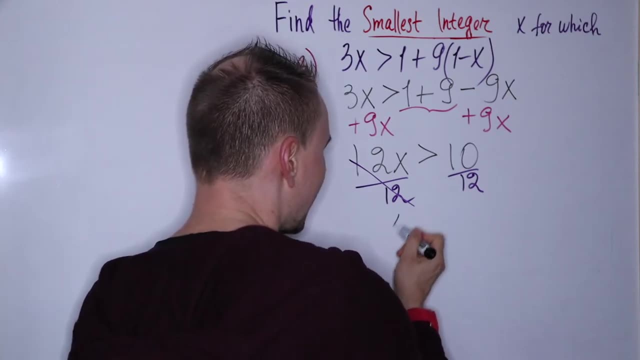 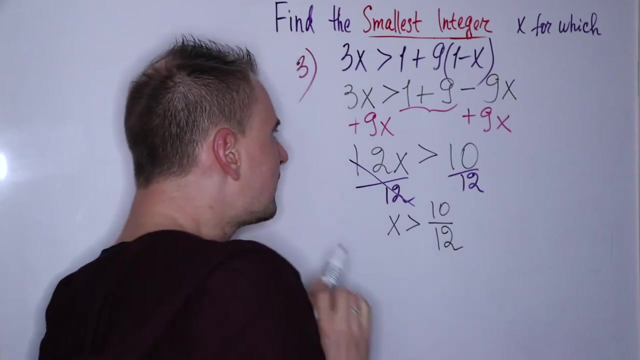 Divide through both sides, So divide out by 12. So 12 goes away, disappeared bye-bye. So you are left with x greater 10 over 12. And again both top and bottom happen to be an even number. 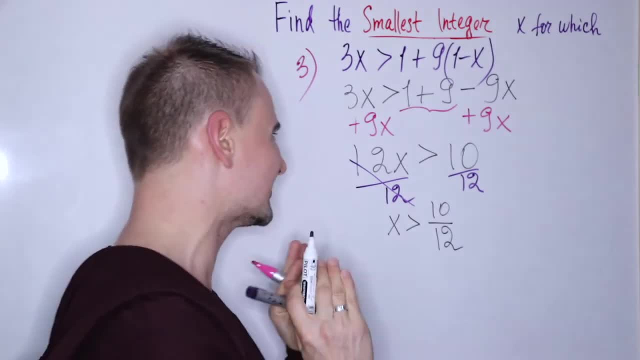 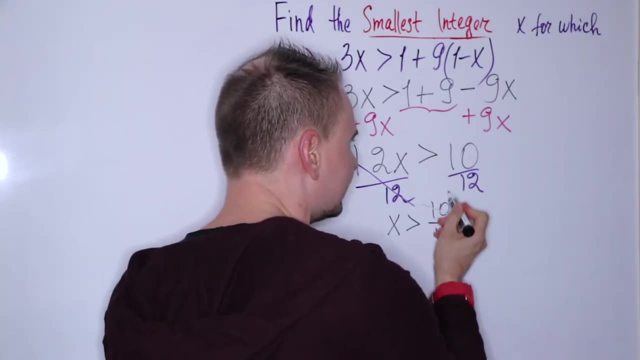 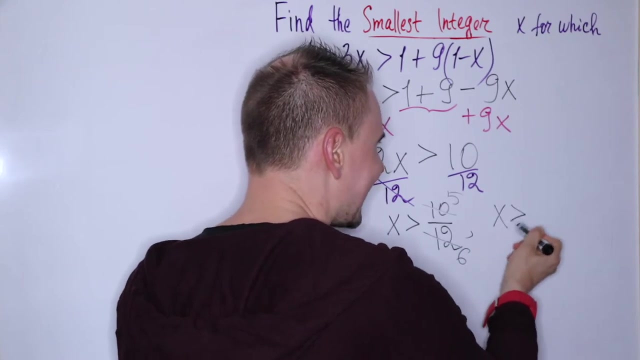 So try to reduce, Try to reduce it as much as you can, So at least this fraction can be reduced by 2, since 2 goes into 10 five times And 2 fits into 12 six times. So you would be left with x greater than 5 over 6.. 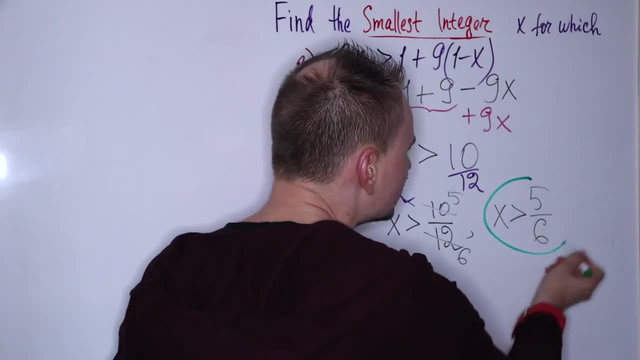 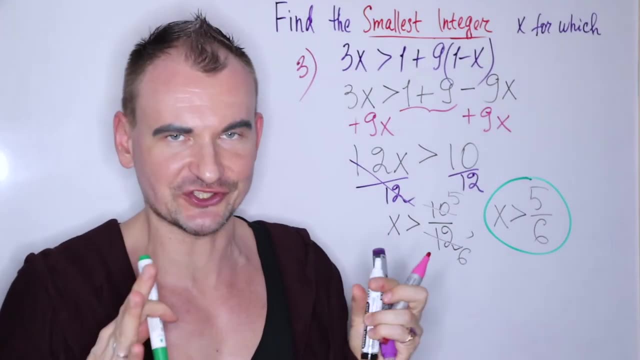 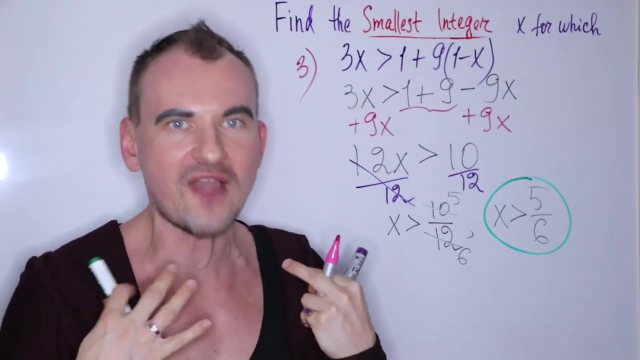 All right, Again at this point, this is your solution set to this inequality. But since we are not after the solution set, basically we are looking for after the smallest integer number, The smallest integer value of x that satisfies, that works for your inequality. 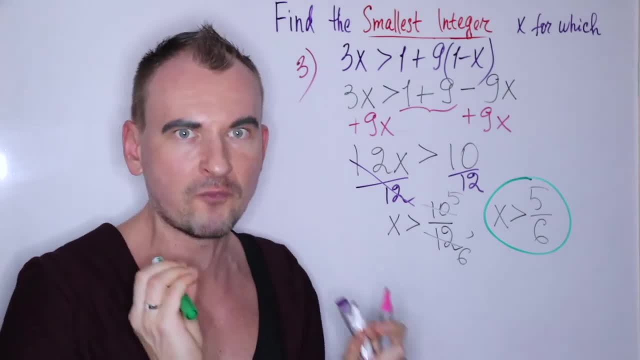 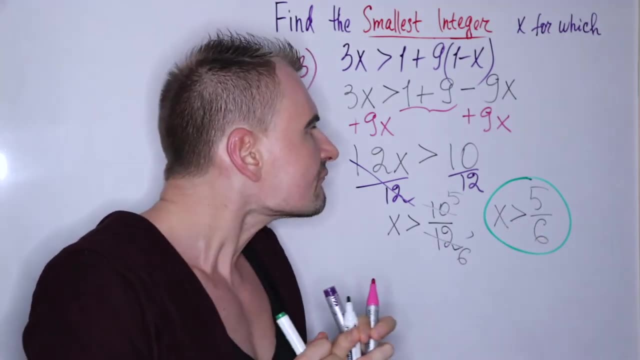 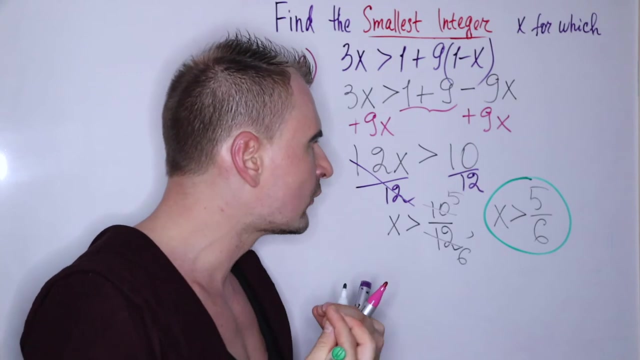 So ask yourself what integer, so what? the whole integer, the whole number or integer number works for this one, And basically you would figure out that the smallest integer that works for this inequality is going to be 1.. So the smallest integer.